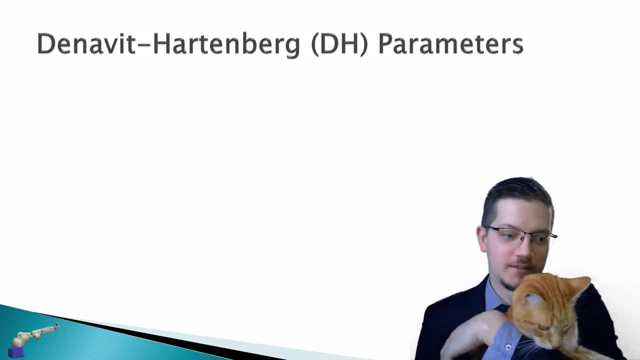 can be described with a minimum number of four parameters, Right? So we have a minimum number of four parameters applied in sequence. We rotate about the z-axis by theta. So in our first transform we have a rotation about z by theta. We translate: about the z-axis by d. 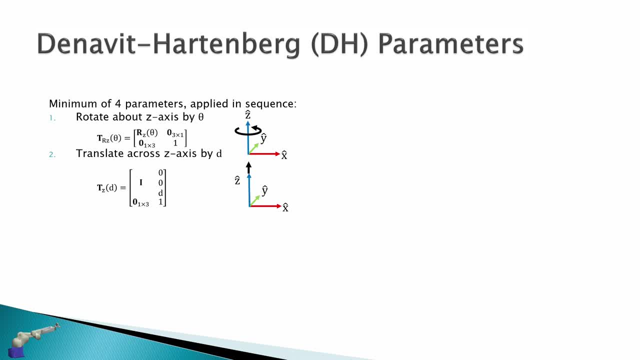 So in our second transform we replace the z-component with the variable d. in the translation vector, The third one, we translate across x by a variable a. So in our third transform the x-translation component is given by a. And then, lastly, we rotate about the x-axis by alpha. 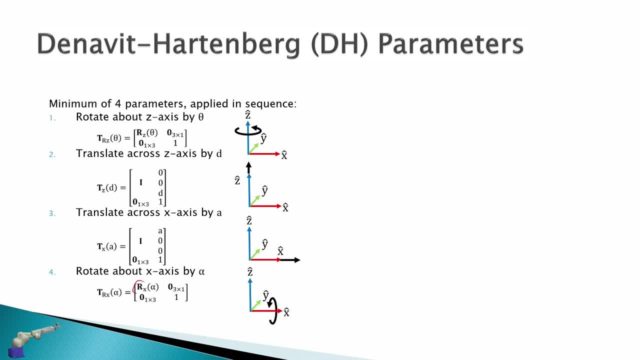 So in our last transform we have a rotation about x by angle alpha. So for our joint frame J-1 to J, we have the concatenation of all these transforms. So first a rotation about z by theta, A translation about z by d. 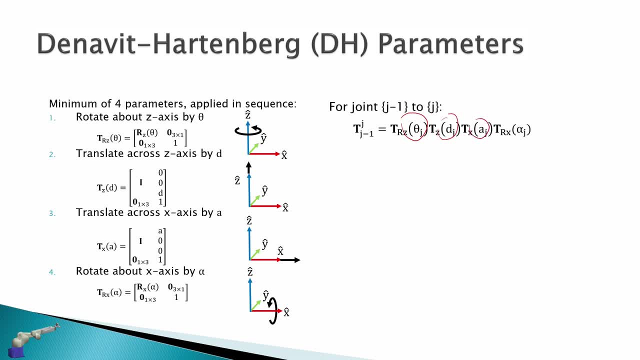 A translation about x by a And a rotation about x by alpha, And therefore to get the forward kinematics from frame 0 to frame n, Then we just multiply all of these together, So we have J-1 to J for every joint, J up to n joints. 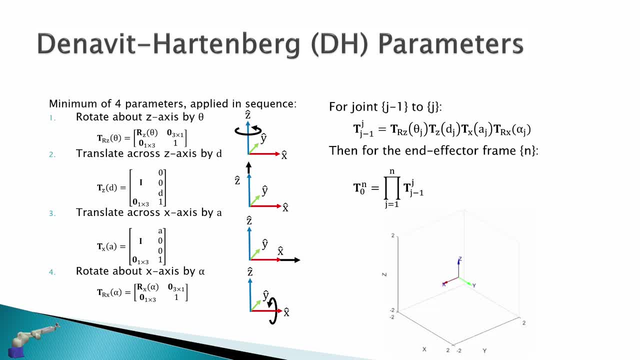 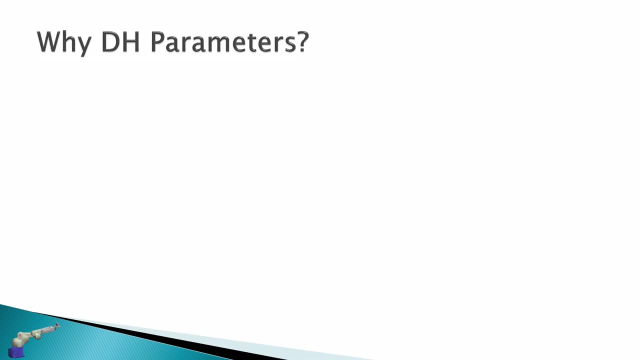 And we multiply all of these together. So here is a nice little animation showing what it looks like. We rotate about z, Translate about z, Translate about x And then rotate about x. So why do we use the d-h parameters? Well, firstly, it's the minimum number of parameters needed to describe forward kinematics. 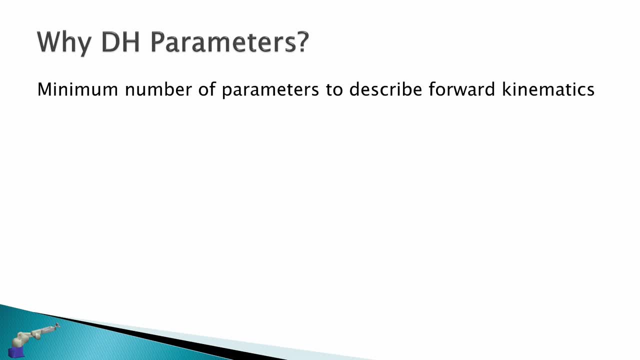 So we could define any kind of transformation matrix between frames, But d-h parameters are the most efficient. It also allows us to use universal nomenclature. So knowing the d-h parameters gives complete knowledge of the kinematics of a robot And also it's easily understood by anyone. 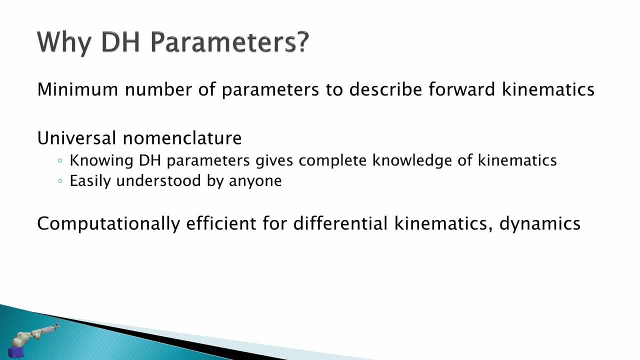 And then it's also computationally efficient for the differential kinematics and dynamics. So we need to minimize the number of calculations for high frequency feedback control. So even though we have super powerful computers, this can still add up, Especially when we have lots of sensors. 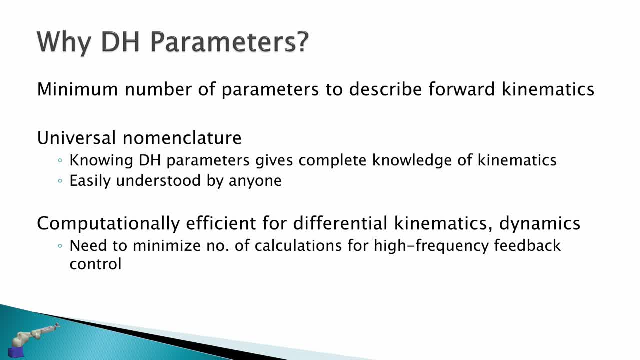 lots of vision processing really complex robot structures, So we need to minimize the computational cost for our robot control. And consider that electricity travels 3000 kilometers in 0.01 seconds at 100 hertz, So this is a huge distance in such a small amount of time. 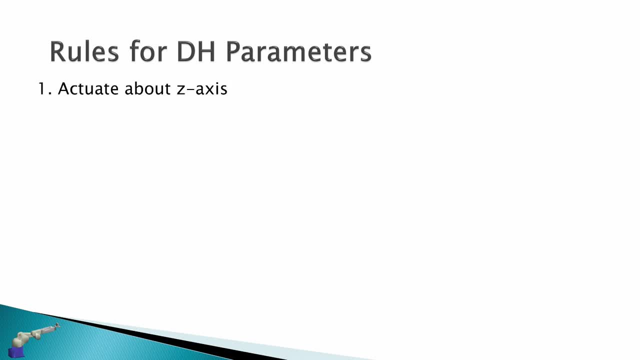 So there are rules for applying d-h parameters. The first is that we actuate about the z-axis. So for a revolute joint we just rotate about z, like shown. So in our first transform, if we have a revolute joint, we replace theta with q. 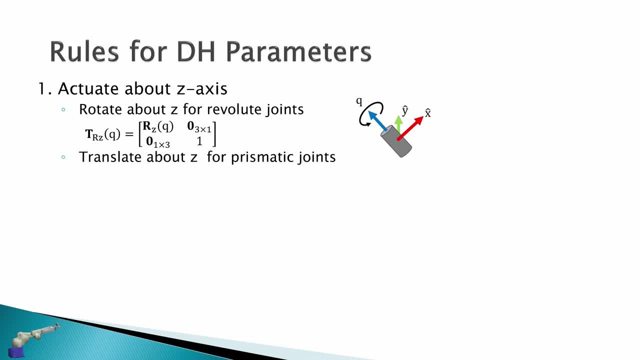 And if we have a prismatic joint, we translate about z. So our second transform: we replace the z component with q, Right, so we only actuate about z. Second, the axis for z is perpendicular to and intersects the axis for x of frame j. 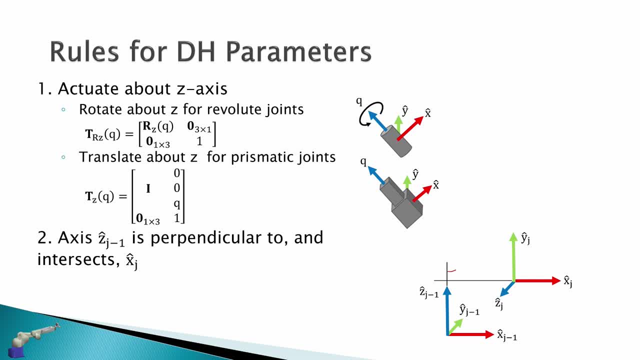 So, as you can see in the diagram here, these two axes projected will intersect and they're at 90 degrees to each other. Lastly, we don't need to define the y-axis. This is just solved implicitly, So the y-axis will just be. 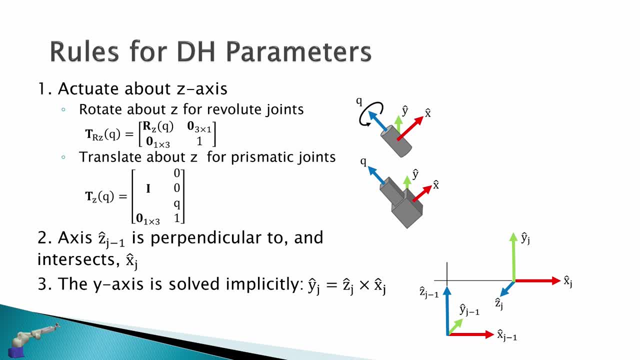 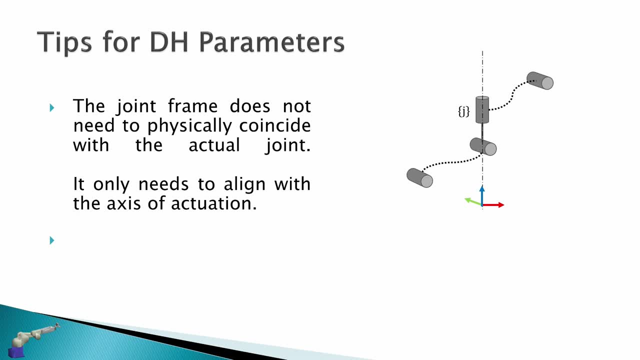 the cross product of z and x Right. so here are some tips for d-h parameters. Firstly, the joint frame does not need to physically coincide with the actual joint. It only needs to align with the axis of actuation. So in this depiction here, 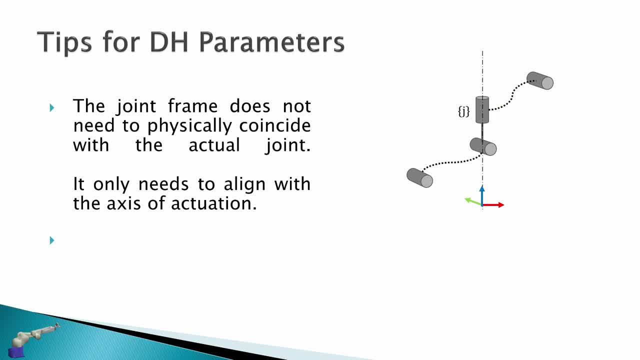 we can see that the physical joint might be up here, but the frame of reference for this joint can be anywhere along this axis Right, it could be anywhere here, It doesn't need to be on the actual joint. Second, the robot arm can be arranged in any configuration that suits the d-h parameters. 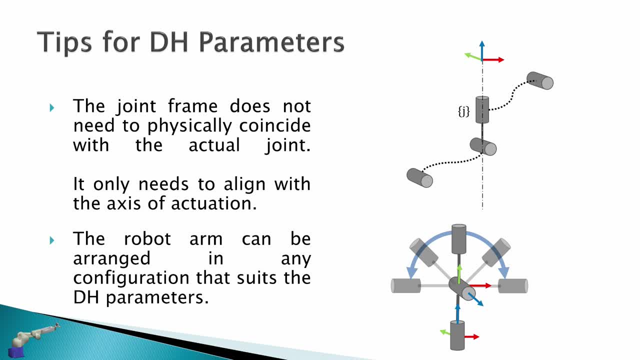 So the robot configuration should suit the d-h parameters, not the other way around. So we can put this joint here in any location around its previous joint, But we just pick the one that suits the d-h parameter configuration And that would be in this location here. 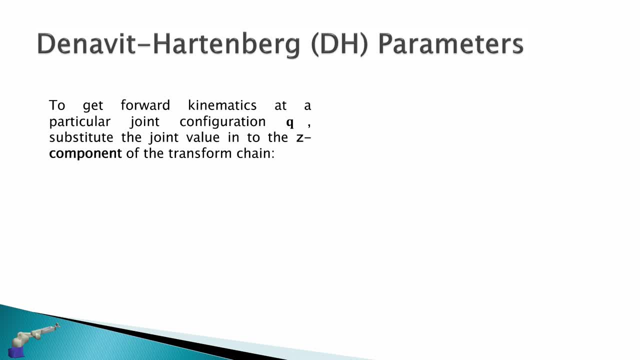 Right. so to get a forward kinematics at a particular joint configuration q, we just substitute the joint value in the z component of the transformation chain, So the transform from frame j-1 to j. if we have a revolute joint we just substitute the rotation about z with the joint variable q. here 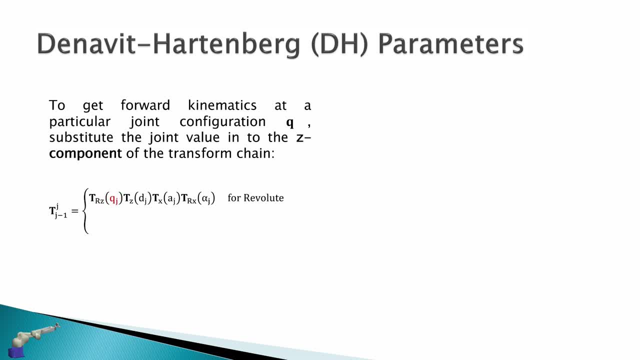 And for a prismatic joint, we substitute the translation component about z with our joint variable q. Now alternative sequences can be used for d-h parameters, and this is one that I made up, so it might not be 100% accurate, but it illustrates the point. 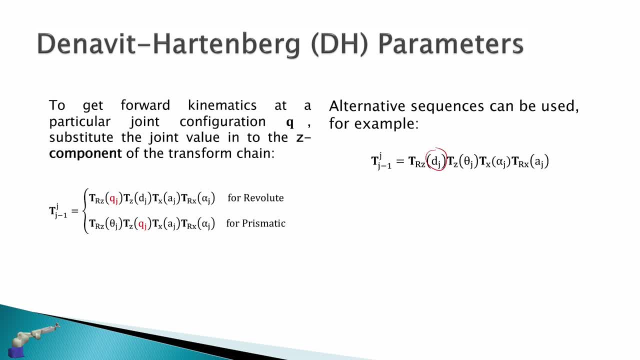 I had d theta alpha a, But the important point is that we must use the same sequence. Matrices are not commutative And so use the same sequence for all joints. So different textbooks will give different combinations of d-h parameters. 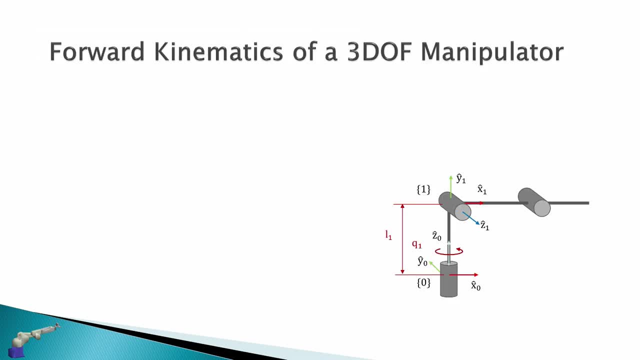 You must use the same one and specify which ones you have used. So let's return to our 3DOF manipulator that we looked at for the forward kinematics in the previous lecture. So the d-h parameters from frame 0 to 1: 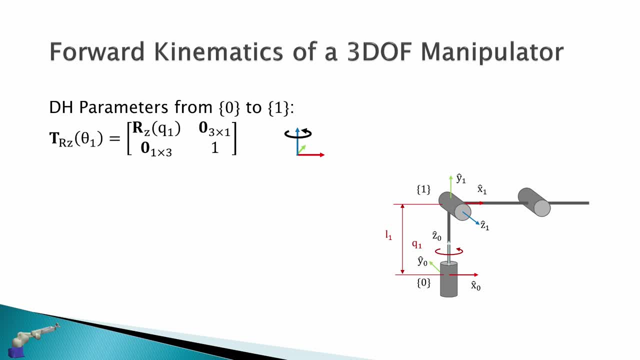 is first given by a rotation about the z-axis, by q1.. So this is our variable, q1 for this joint, and we're rotating about the z-axis. So our first transform will be given by this matrix here, And then we want to move up the z-axis. 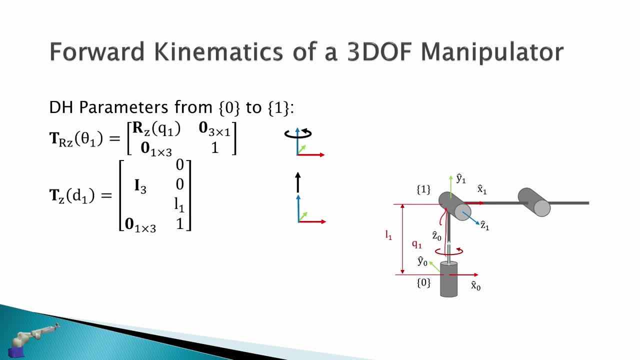 So to get to the next frame we have to move up by l1 the distance of this link length here. Then the next one will be a translation about x by a. But you can see that there is no offset between these joints, and so a will be 0.. 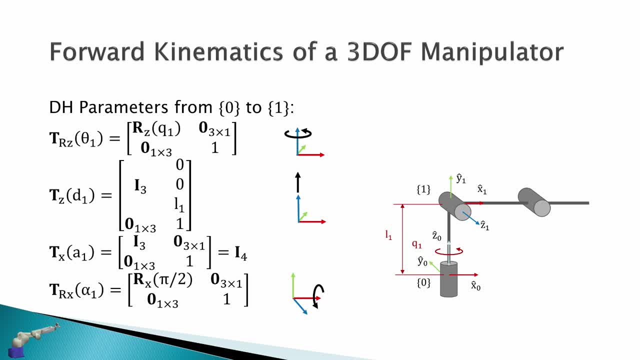 And lastly, we have to rotate about the x-axis by alpha. So to get this z-axis here to align with this z-axis here, we rotate about x by pi on 2.. Now we want to get from frame 1 to 2.. 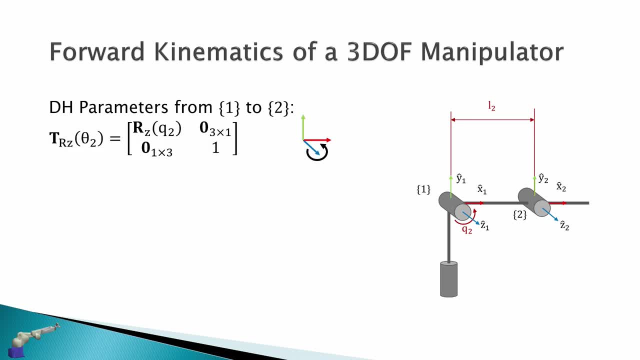 So again we have a revolute joint and we rotate about the z-axis. So this is our variable: q2 about the z-axis z1. So we just substitute q2 into a z-rotation matrix. Then the next would be a translation about the z-axis. 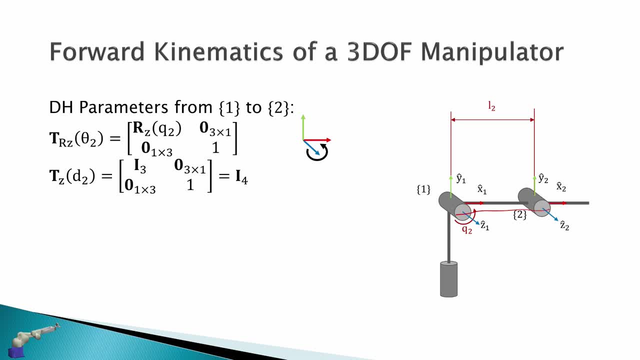 but you can see that these are not offset in z, So therefore we have 0.. Then we have a translation about x. So to get from here to here, we translate by the link length l2.. Then the last would be a rotation about x by alpha. 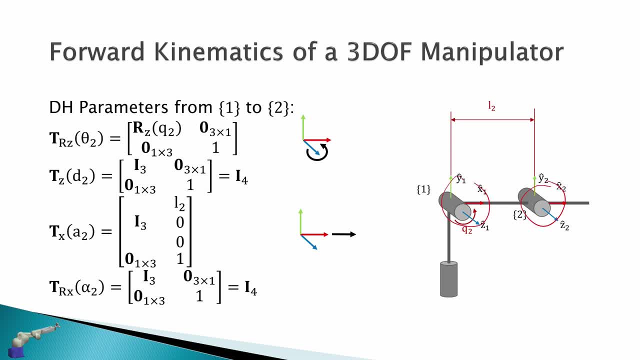 But you can see that these two frames are already in alignment, And so, therefore, we have 0 rotation, which will give the identity matrix. Then, lastly, we go from frame 2 to 3. And so, again, we rotate about z here, q3. 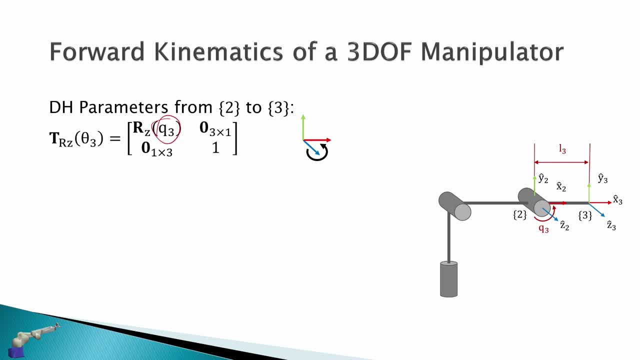 and therefore we substitute q3 as our variable theta. We translate across the z-axis by d3, but again because these are not offset in z, therefore this is 0.. The next will be a translation across x by a, And so we have to move along the x-axis. 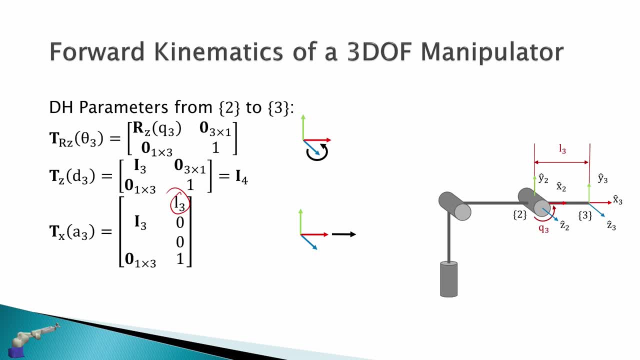 and this is just the link length l3 for the x component. And then, lastly, will be a rotation by alpha about the x-axis, But again, these frames are already in alignment, So this alpha will be 0, which gives the identity matrix for a rotation about 0.. 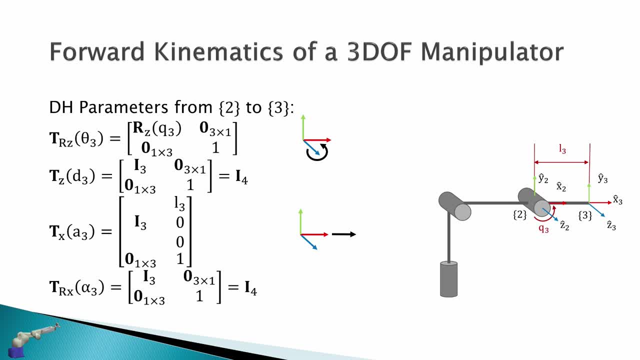 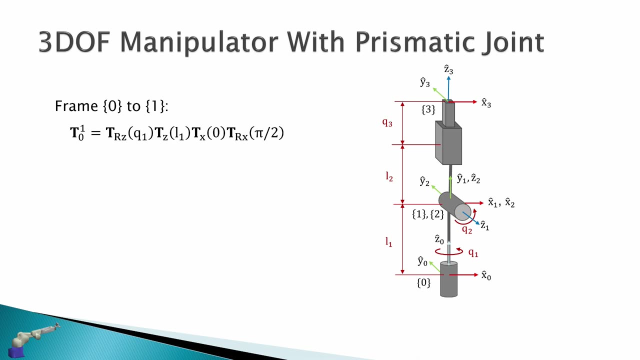 Right. so therefore we have solved all the transforms from j-1 to j of our 3-link manipulator. So let's consider this 3-DOF manipulator with a prismatic joint. So from frame 0 to 1, it's the same. 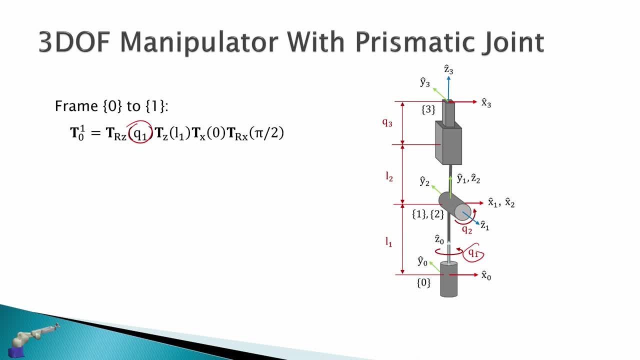 We have rotation about the z-axis by q1, translation up z by l1.. We don't need to translate about x, so this will be a 0. And then we have to rotate by pi on 2 to get the two frames in alignment. 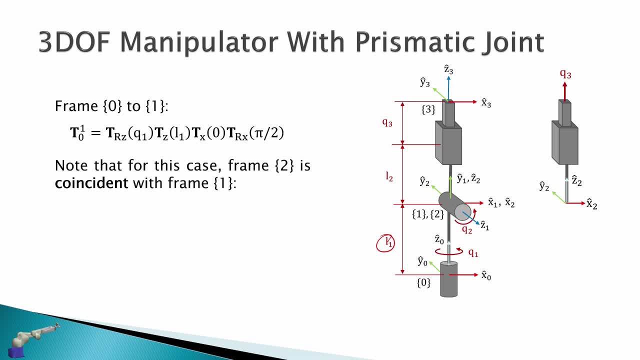 And note that for this case, frame 2 is coincident with frame 1.. So we had before I described that the frame of reference for a joint does not need to be located on the physical axis and therefore to perform the dh parameters on this type of structure. 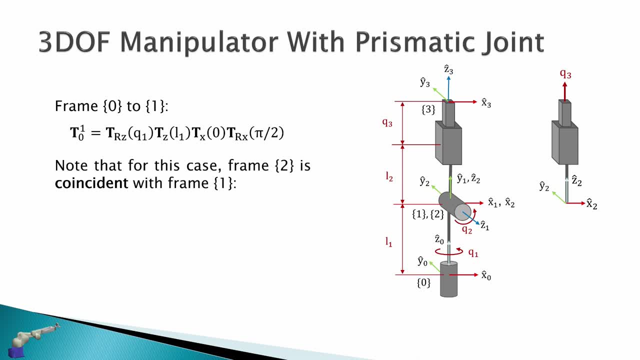 the frame for this joint here must be located down here, coincident, Otherwise the dh parameters won't work, and this is fine, It still works out mathematically. So 1 to 2, so we're at frame 1 and we're going to frame 2. 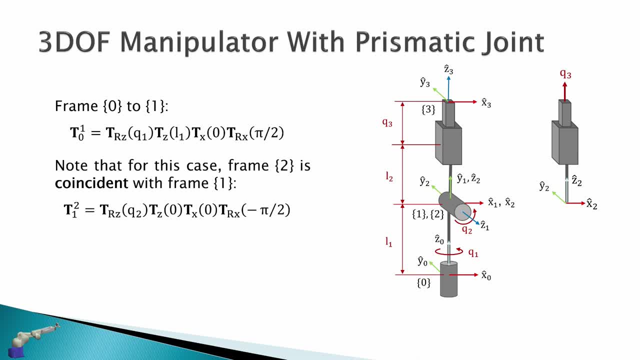 and they're in the same location Again: q2 about z1.. They are coincident, so we have no translation about z and no translation about x. But now we need to rotate back by pi on 2 to get this z axis pointing up. 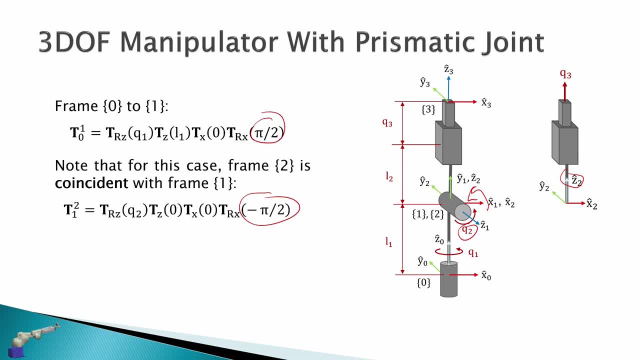 So negative pi on 2. to cancel out this pi on 2 here- And since frame 2 is not located on joint 3, so this frame is not up here where the physical origin of the joint would be- we need to add the link offset for the z translation. 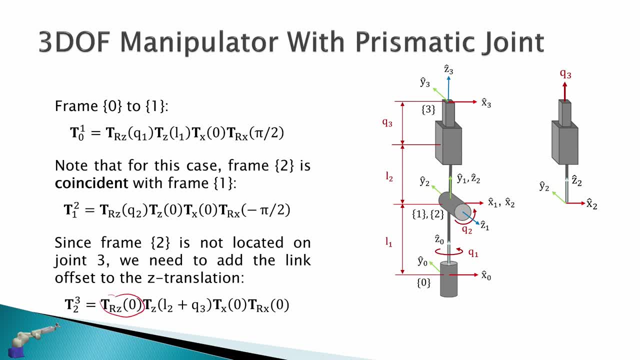 We start with a rotation about z, but we don't need to rotate about z, So this will be 0. And we translate across z by l2 plus q3 to get from here to here or, more importantly, here to here, And then we don't need to move about the x axis. 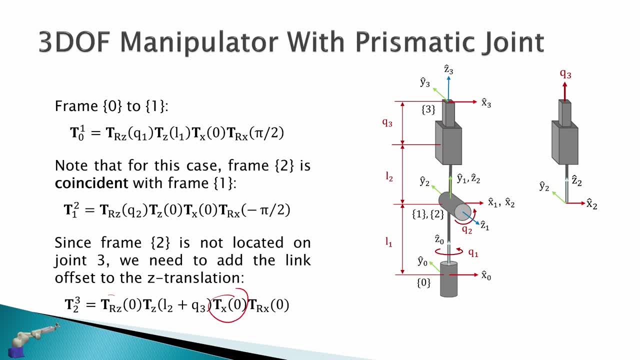 because they're in alignment, so that's 0.. And again, we don't need to rotate about x anymore either, because these frames are now oriented in the same way, So this will be 0.. So this would be an example of how to perform. 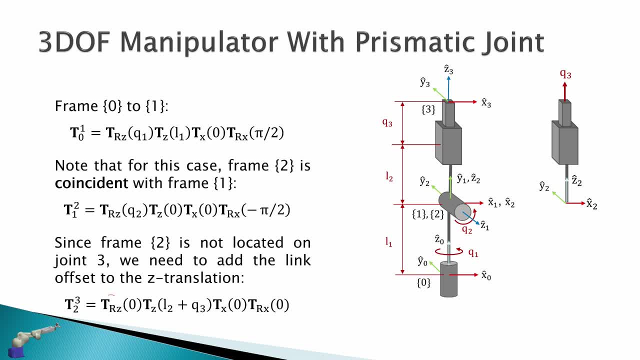 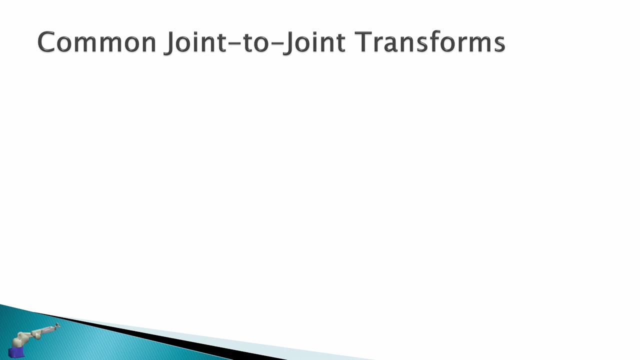 the forward kinematics with dh parameters, where we have some sort of annoying kinematic structure like so. So therefore, frame 1 and 2 are coincident and we account for this offset between frames with our dh parameters here. So I'm going to give you some common joint-to-joint transforms. 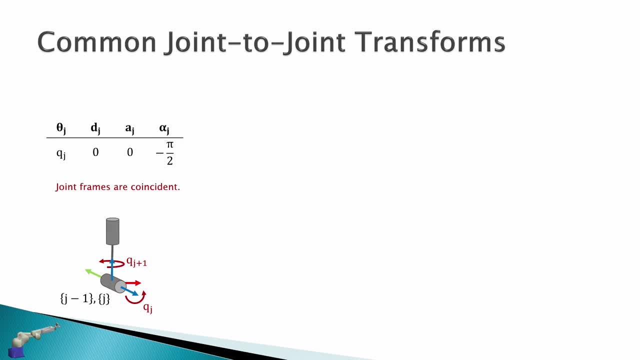 that I have seen in my limited experience. So the first would be exactly what we saw in the previous example. So we have joint frames that are coincident. So when these two joints are perpendicular, we need to specify this joint frame down here at the same point as the previous one, j-1.. 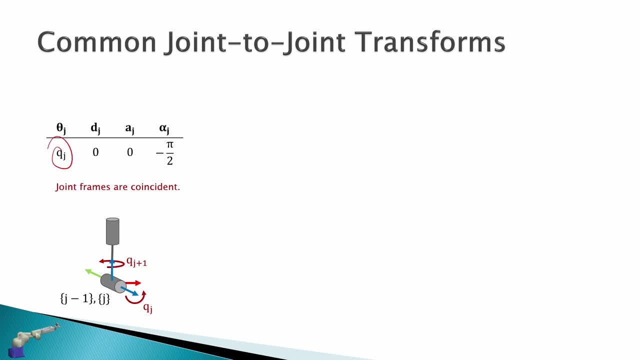 And therefore we have a rotation about z by q. No translations at all, And we just do a plus, minus pi on 2 to get the z axis of j pointing up. The next would be this kind of arrangement. So we have z rotation with q. 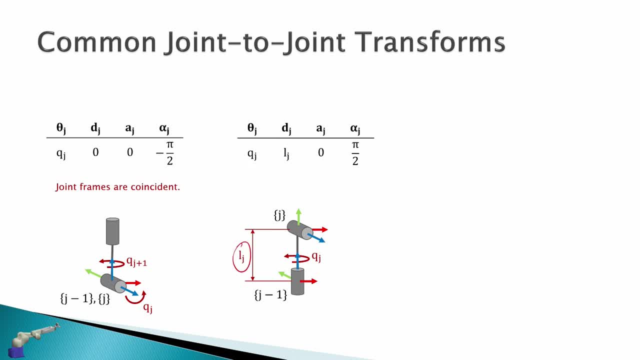 Translation up z by the link length. here, No translation about x, because they're in alignment. And then we have to rotate about pi on 2 to get the z axis pointing this way, which is orthogonal to this one. And lastly, this really simple arrangement.